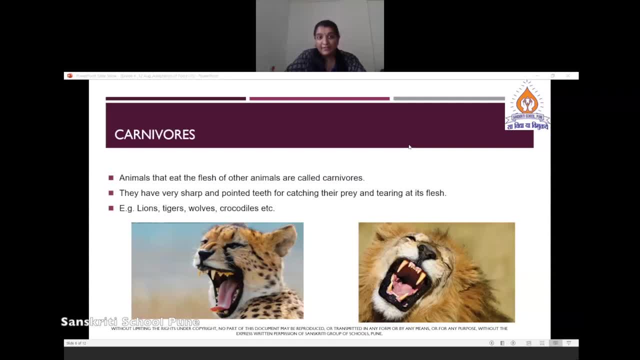 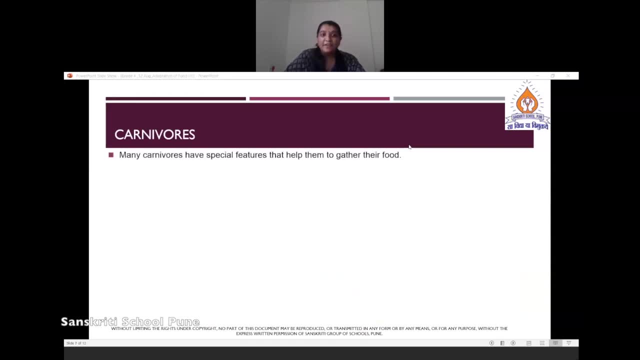 Examples are lions, tigers, wolves, crocodiles, etc. Many carnivores have special features that help them to gather their food. Birds such as eagles and kites have sharp claws and strong hooked beak to tear at the flesh of their prey. 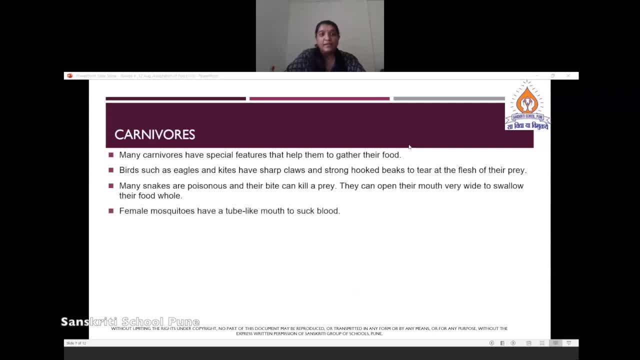 Many snakes are poisonous And they are very poisonous And their bite can kill a prey. They can open their mouth very wide to swallow their food as whole. Female mosquitoes have tube like mouth to suck their blood. Let's move on to the next category. 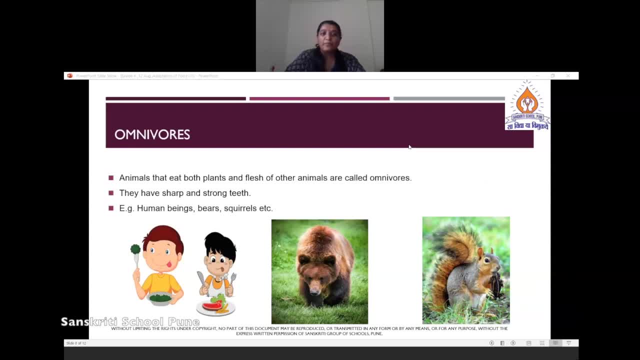 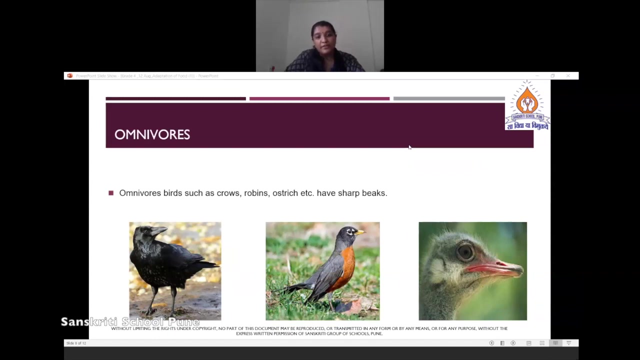 And that is omnivores. Animals that eat both plant and flesh of animals Are called omnivores. They have very sharp and strong teeth. Human beings, bears, squirrels are few examples of omnivores. Omnivores birds such as crows, robin ostrich have very sharp beak. 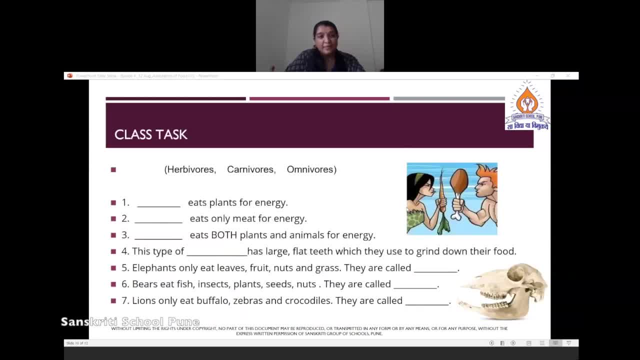 So let's come to the class task. Here you are going to fill in the blanks with the help of the words given in the bracket, And the words are herbivores, carnivores and omnivores. So let's start. I will read each question for you all. 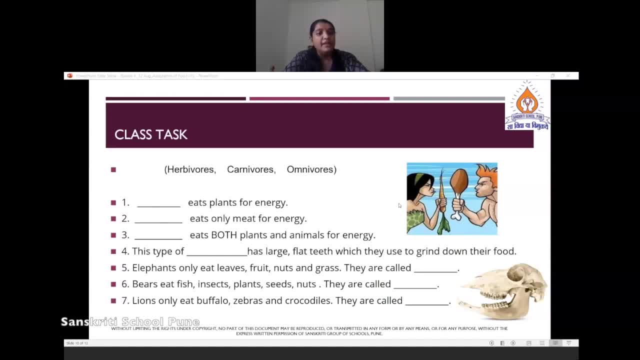 Question number one: Dash eats plants for energy. Question number two: Dash eats only meat for energy. Question number three: Dash Dash eats both plants and animals for energy. Isn't this easy, I think, so You must have got it by now. 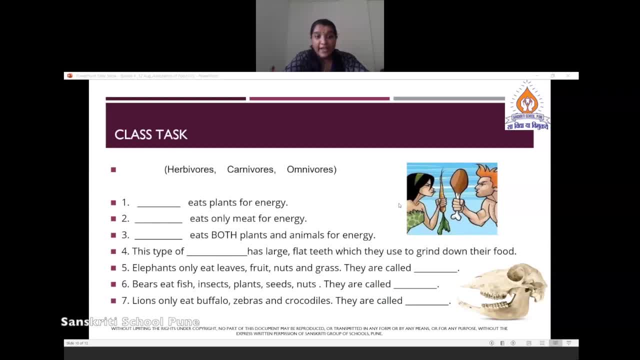 Question number four. This type of dash has large flat teeth which they use to grind down their food. So which one of these three Think? Question number five: Elephant only eat leaves, fruits, nuts and grass. Question number five: Elephant only eat plants and grass.